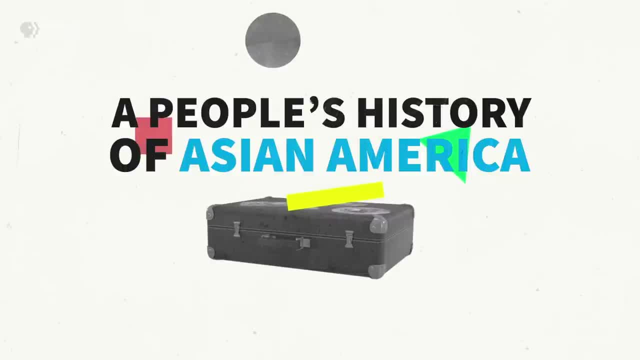 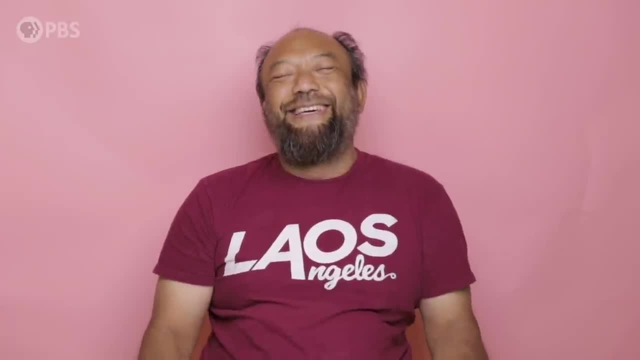 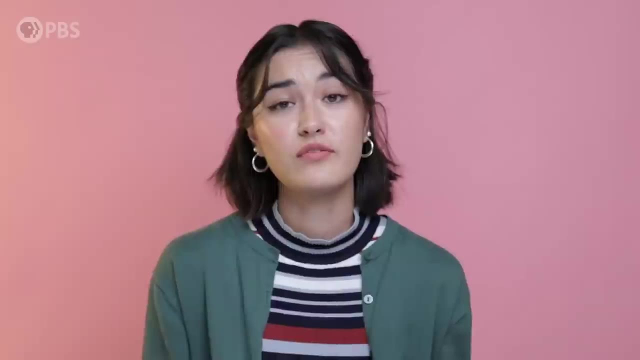 Welcome to A People's History of Asian America. Do I think the term Asian American includes me? I? I yes, I'm kind of torn with that. I feel like it mixes race with citizenship or nationality, If I do choose to be a Japanese. 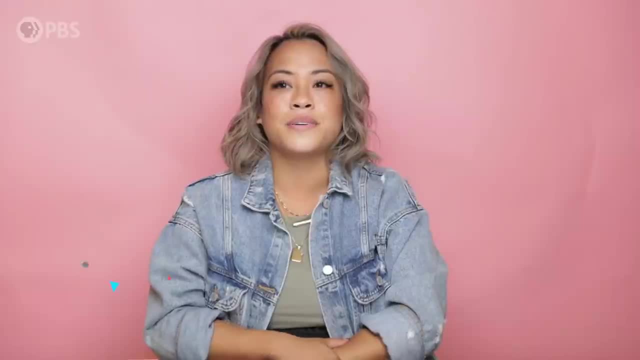 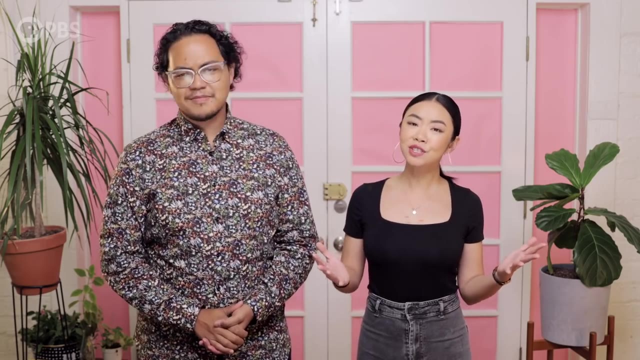 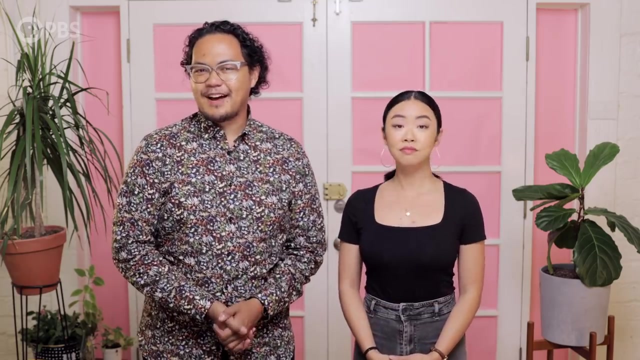 citizen. does that mean I'm no longer Asian American? I don't gravitate towards that term first. I tend to gravitate towards Filipino American first. Prof, do you consider yourself Asian American? Asian Canadian, Pacific Islander? I'm actually none of the above. I'm Ilocano, from Toronto, See. my family and I are from the Philippines. 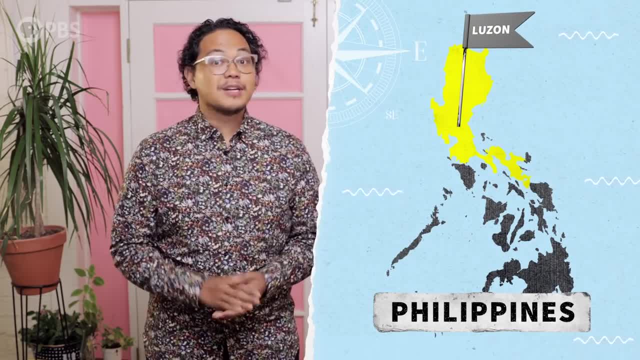 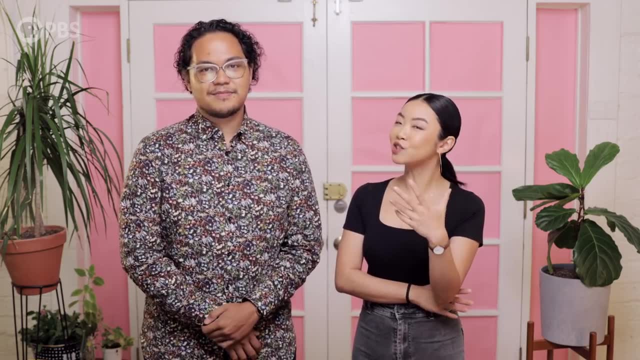 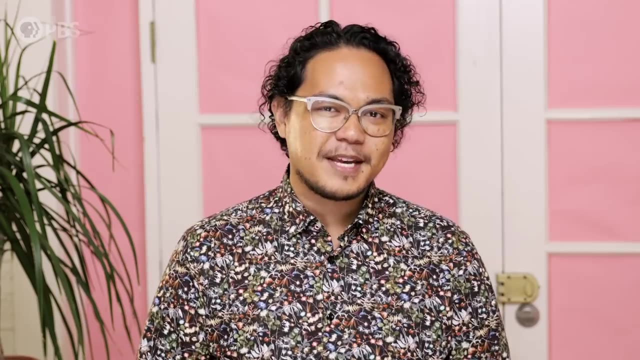 My mom's side is from a region called Northern Luzon, So culturally we're called Ilocano people. Ooh, that's interesting, But how do you explain that to like most people? So my easy answer is that I'm Filipino And, being from Canada, we don't really have this concept of 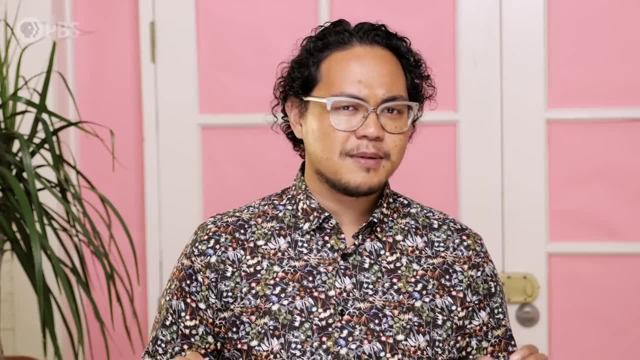 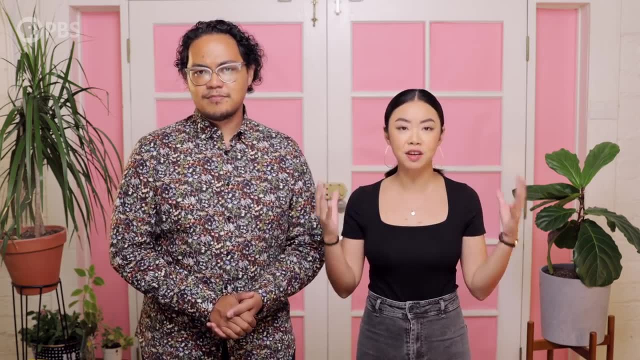 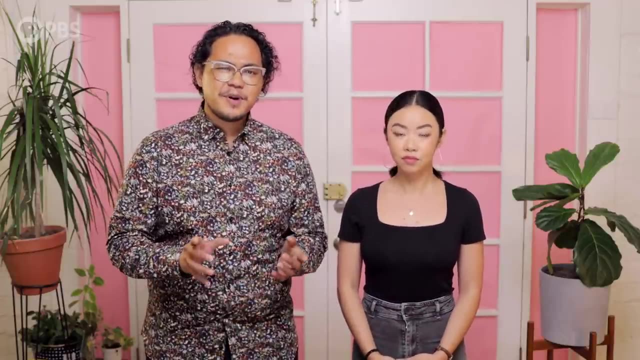 Filipino Canadian, the way that y'all have it down here with Filipino American. That's a pretty crazy concept for me to wrap my mind around, as someone who grew up with everything being hyphen American. Why are there no Filipino Canadians? Well, it has something to do with the fact that the US has ethnic studies and Canada doesn't. 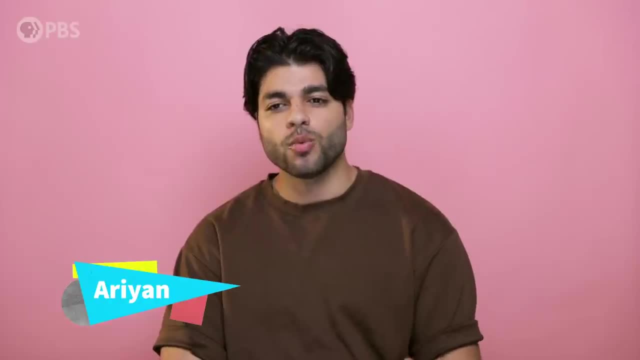 First time I heard Asian American, I didn't know whether it was like a white American term put on us or whether it was us kind of being like: hey, let's form an alliance together so people stop killing us and we can actually have unity between each other. 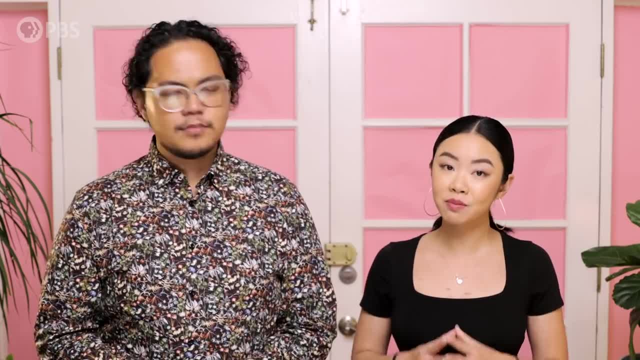 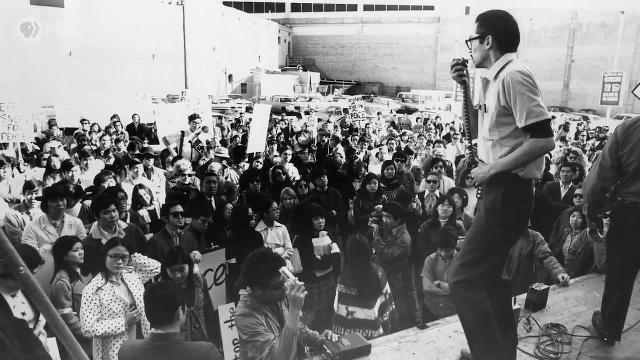 Asian American was actually a chosen term that emerged around the same time that ethnic studies was created as a field. In 1968, inspired by the Black Power Movement, two Berkeley students, Yuji Ichioka and Emma Gee, coined this term: Asian American. 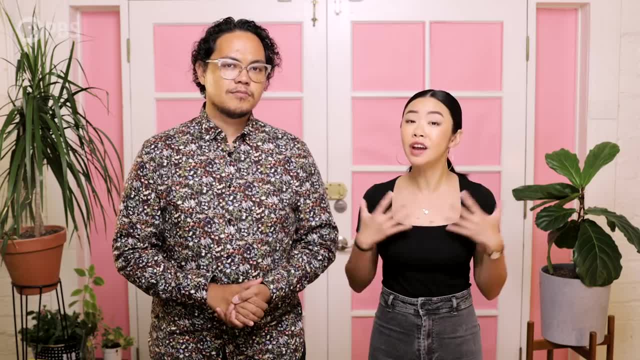 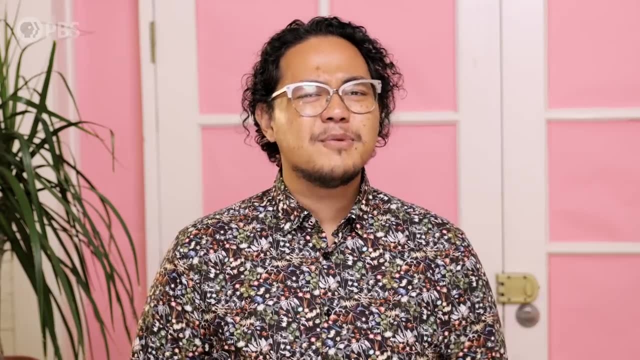 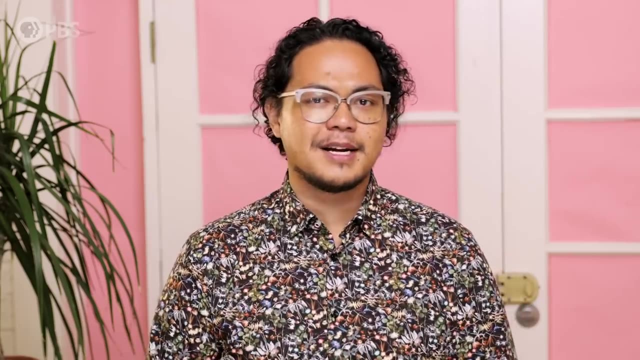 You know, having an umbrella identity that people could unite under does seem pretty powerful. So why all this talk of changing it? Well, maybe we should actually talk about expanding on it. So, as we know, Asian American has its roots in political organizing. So, at its 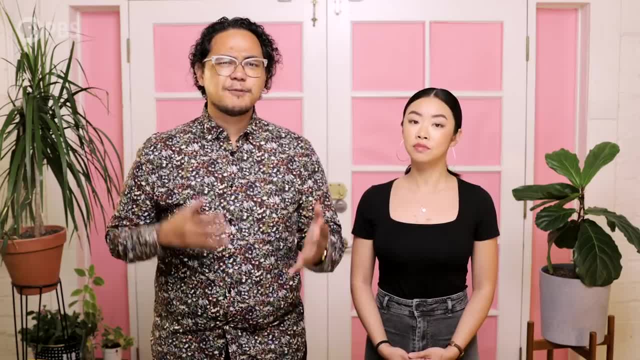 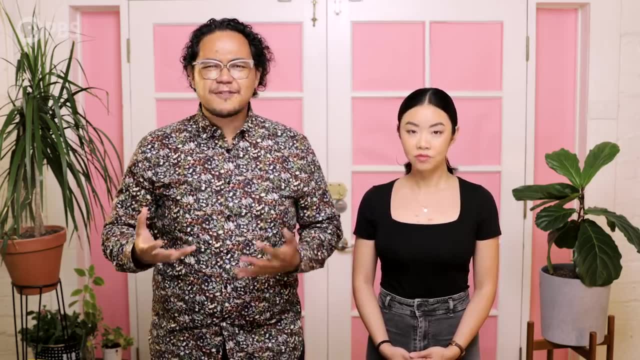 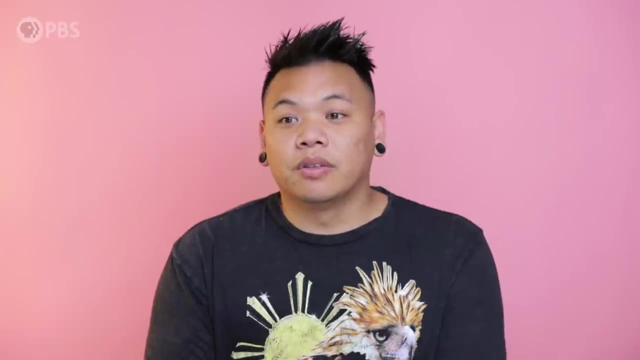 core. it's a political identity. But as this community grows in numbers and geographical diversity and migration histories, the term starts to fall a little short. I don't feel that Asian American all the time includes Southeast Asians or darker Asians. Asia is a. 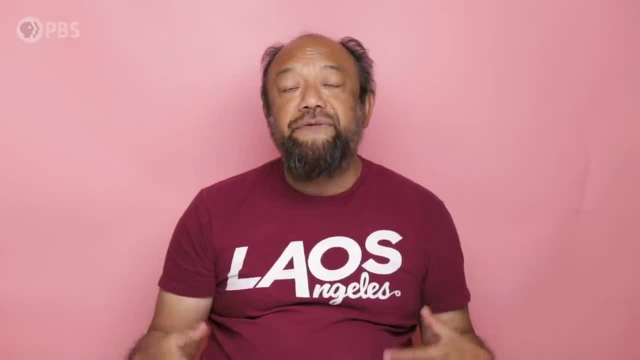 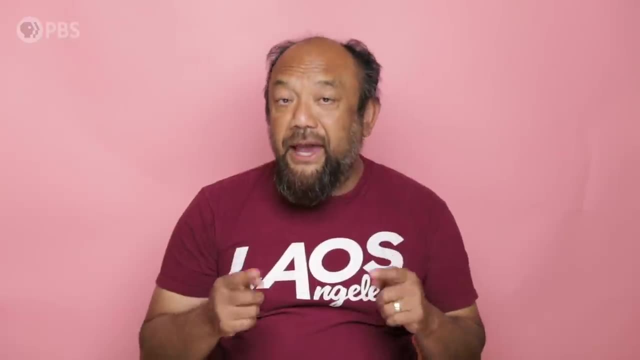 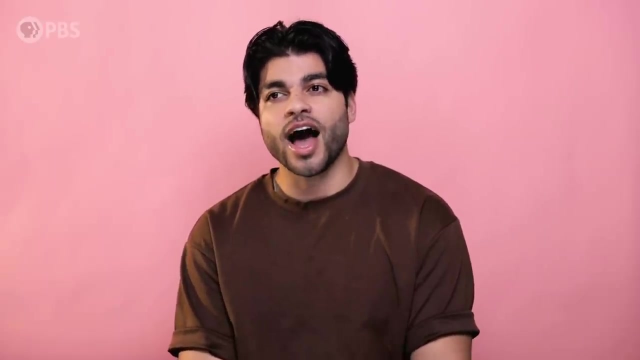 country with so many different nations, different nationalities, different cultures. I do consider Lao and Laotian Americans to be a part of under that umbrella, but as a Lao American I don't feel I'm as represented. The term Asian American, or even South Asian, has been something that I had. 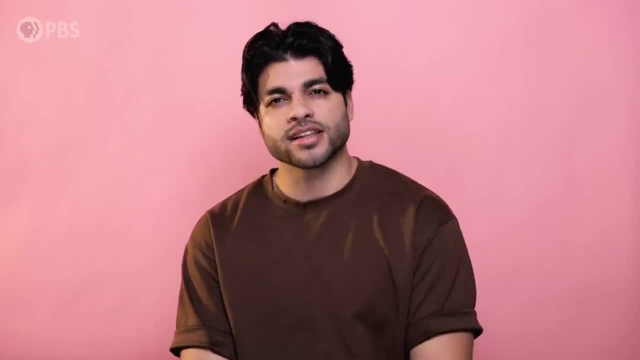 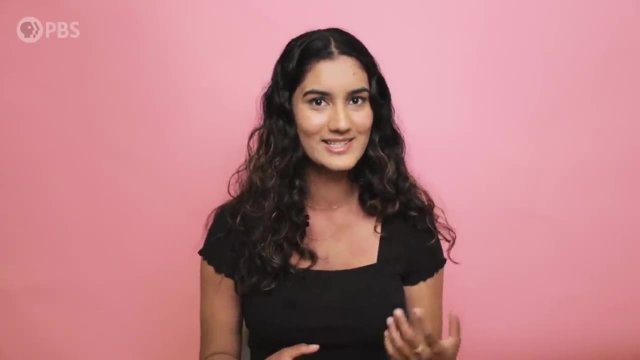 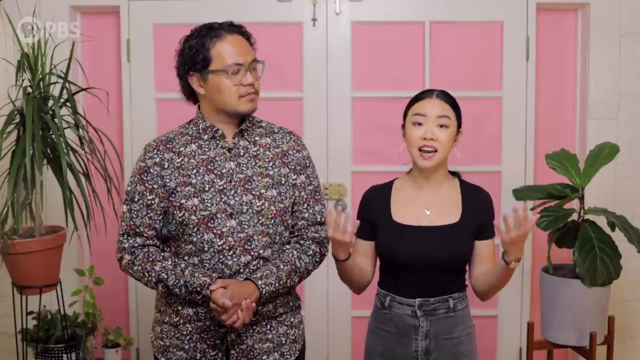 never been associated with growing up in Kenya and South Africa. I think, when we are talking about particularly East Asian experiences, that we should identify them as East Asian, the same way that we identify South Asian experience as a South Asian. Another shortcoming is the way statistics get aggregated under the 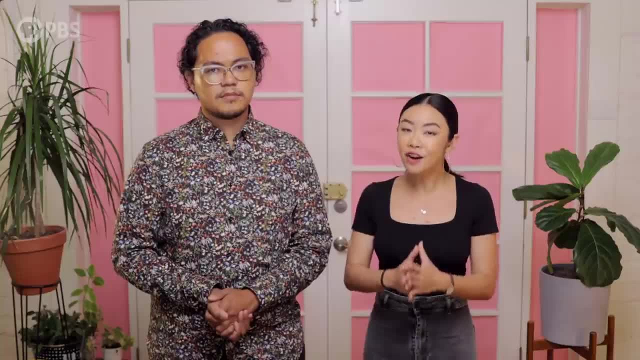 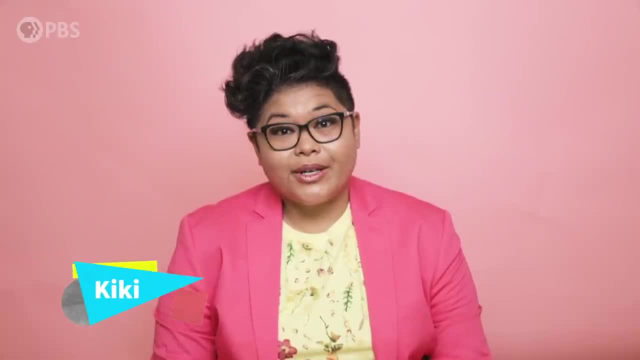 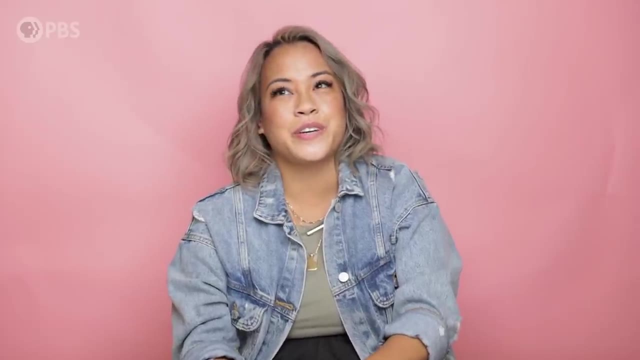 broad term Asian American. Let's take a look at a very common stereotype: that all Asians are crazy rich. The crazy rich Asian stereotype makes me feel really broke. I can say with a complete authority that the crazy rich Asian stereotype has never really been a stereotype. 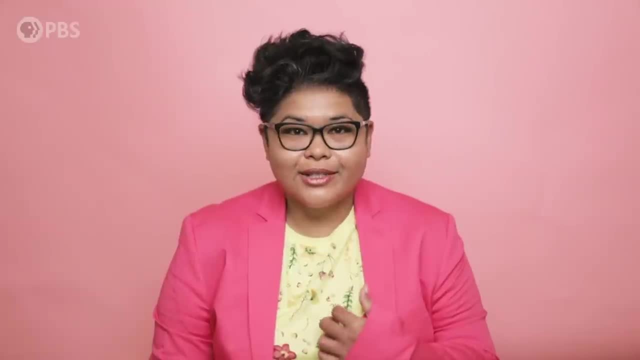 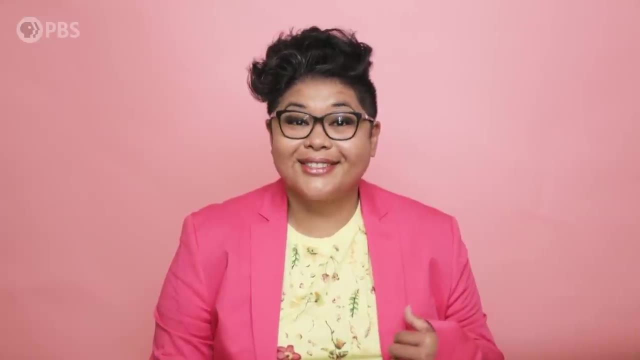 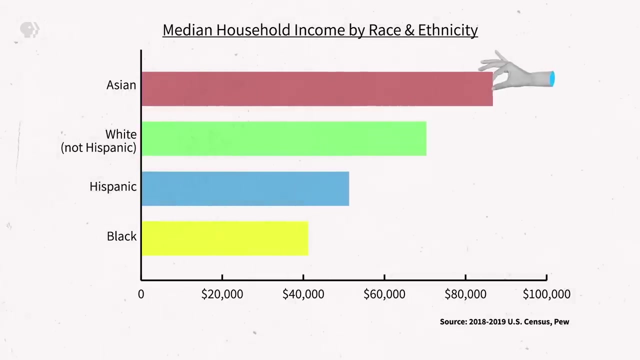 It has never really applied to my lived experience. Myself, as a Pacific Islander, feel like I am wealthy and spiritual, in the spiritual sense though, which you know. that's special unto itself. On paper, it seems like we're doing pretty well economically. 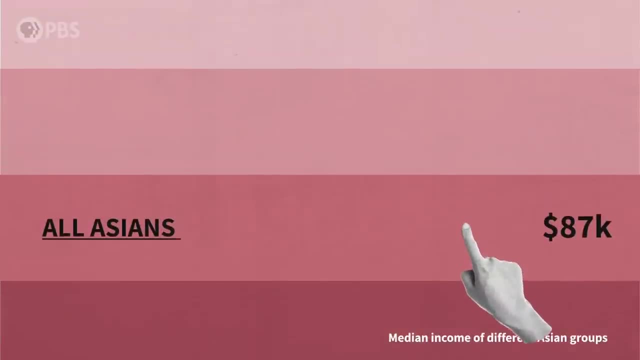 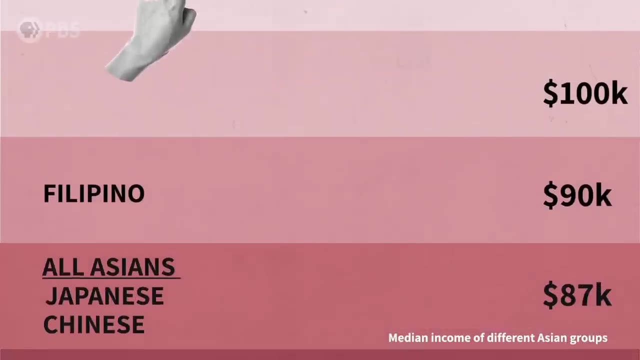 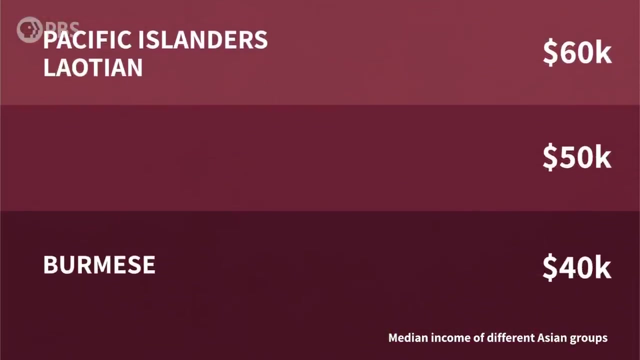 But when you expand on that data, you'll see that the wealth is concentrated among select racial groups, mainly Indian, Filipino, Chinese and African, And when you look at the other end of the spectrum, you'll find Burmese, other Southeast Asian and Pacific Islander communities. 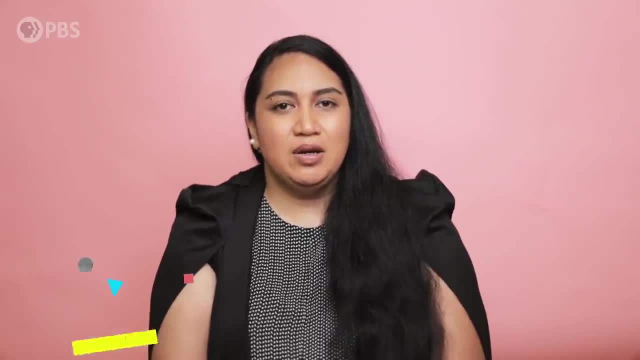 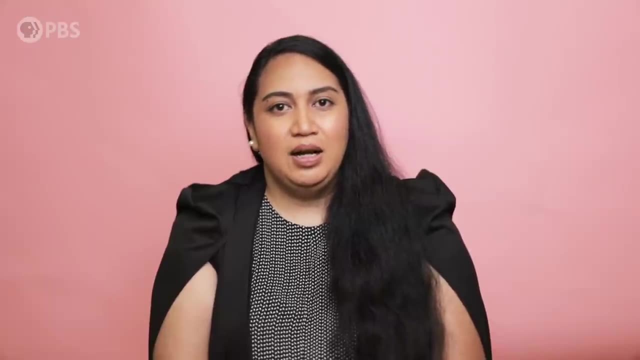 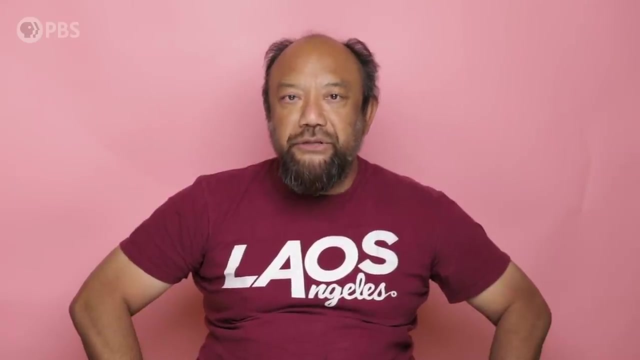 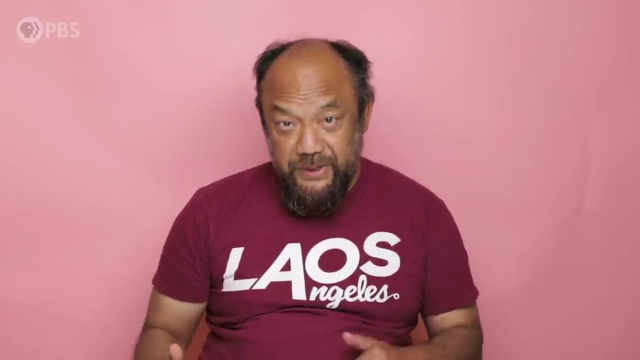 It's important to disaggregate data because we are deemed insignificant and we are deemed too small to be a community on our own as Native Hawaiians and Pacific Islanders or NHPI Lao Americans- majority of them, who came to the US, are refugees, and it is the impact of American engagement in Vietnam that brought me. 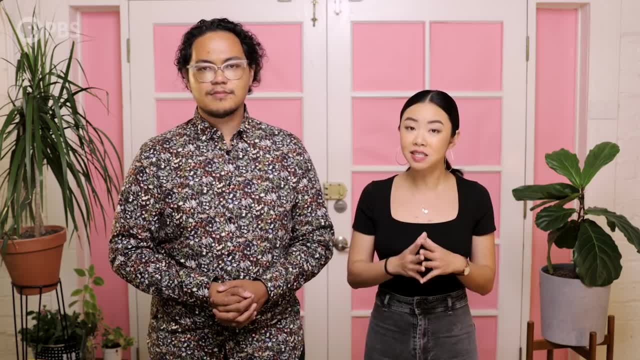 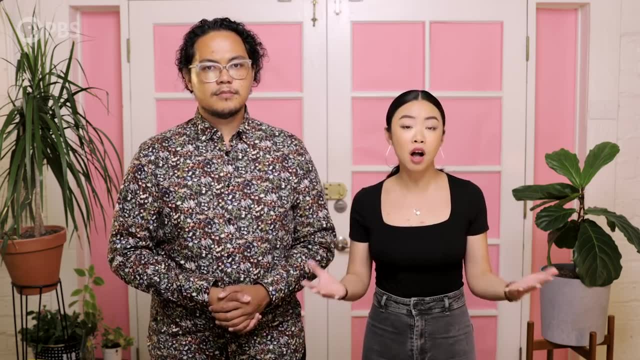 here to this country. What the data hides is the fact that many Southeast Asians arrived in the US as refugees. It also hides the fact that the Pacific Islands, like Guam, the Mariana Islands and Samoa, are still territories of the US which function like colonies. 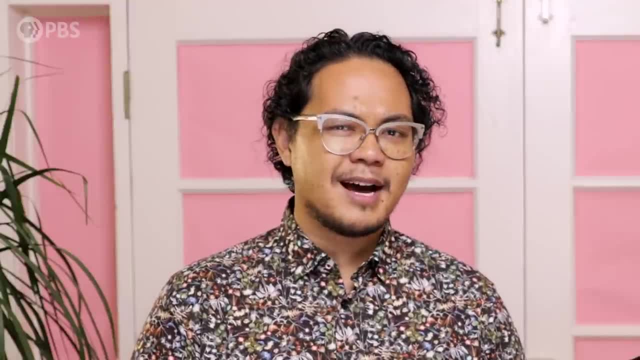 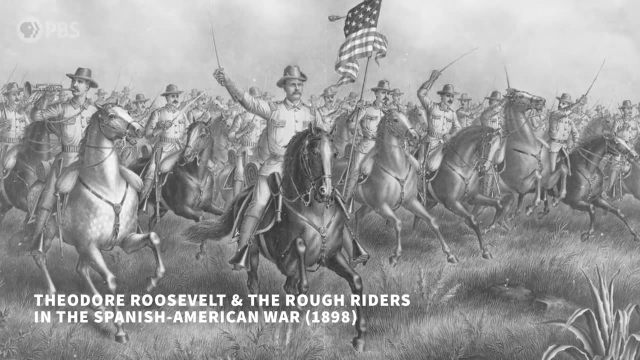 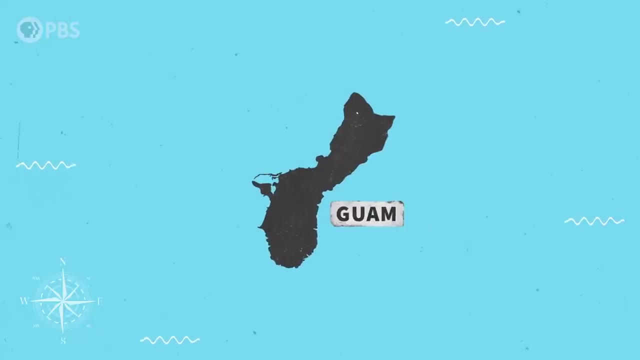 A little history here is important to know. Many of these nations were taken through imperial wars. In 1898, after the Spanish-American War, the United States acquired Spain's island colonies in the Treaty of Paris. After that, Guam, the Philippines and Puerto Rico became US colonies. In that same year, the United States 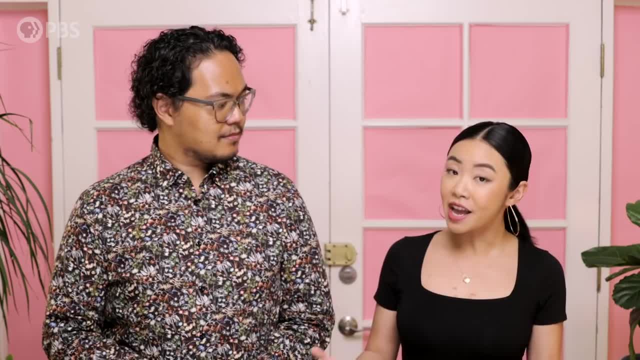 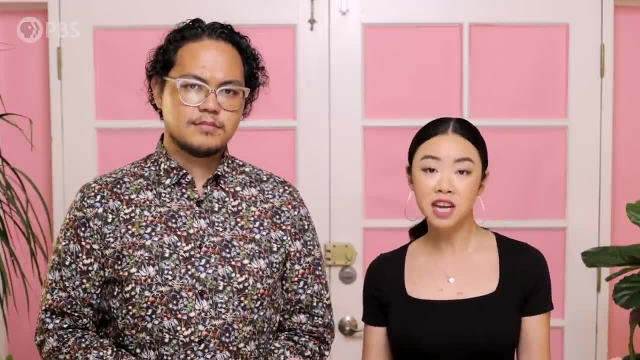 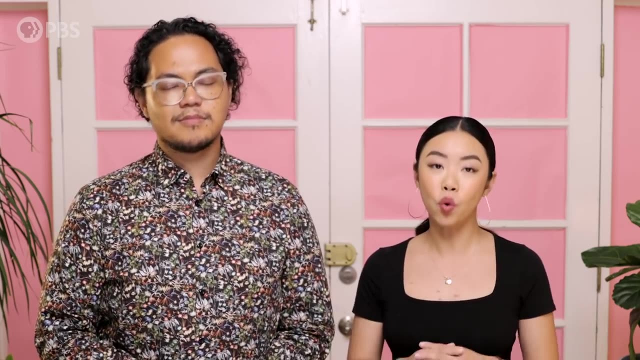 illegally annexed the Kingdom of Hawaii, Which is why, as much of a mouthful as it is, AANHPI is a really important acronym. The histories of Native Hawaiians and Pacific Islanders, as well as Filipinos and other Southeast Asians, is one that's steeped in war and colonization, But these histories. 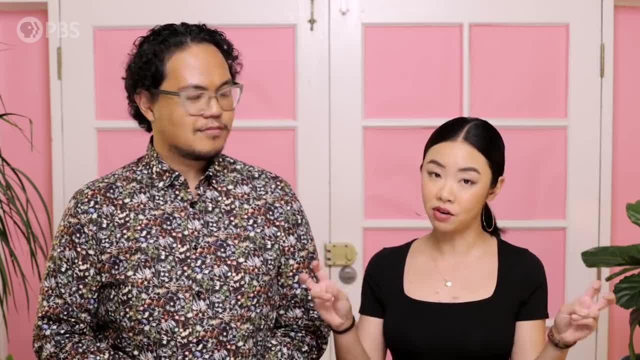 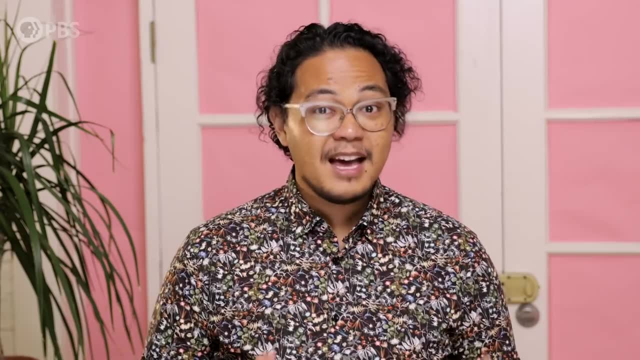 are often rendered invisible under the label Asian American. Let's turn back to you, Adrian. What does it mean to say you're Ilocano from Toronto? For me, I identify as Ilocano first and foremost because it challenges our assumptions. 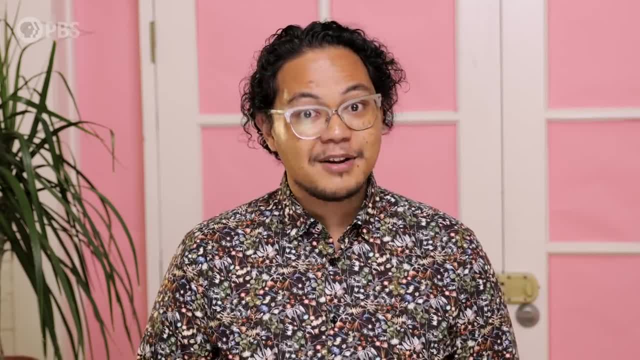 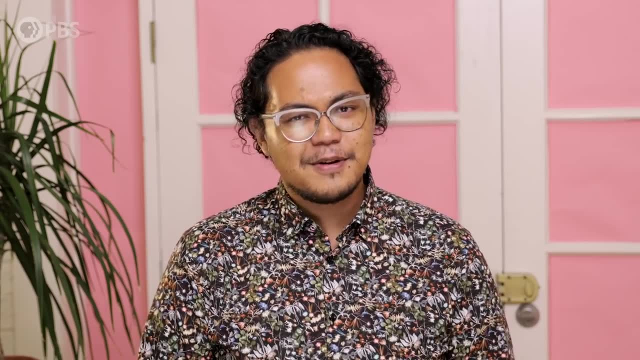 of what being Filipino means, that matter, whatever the heck Asian and Asian American mean. See, it might be easier for me to say Filipino, but the whole point of me telling you about my native land in the Philippines is to make all of us question our assumptions. 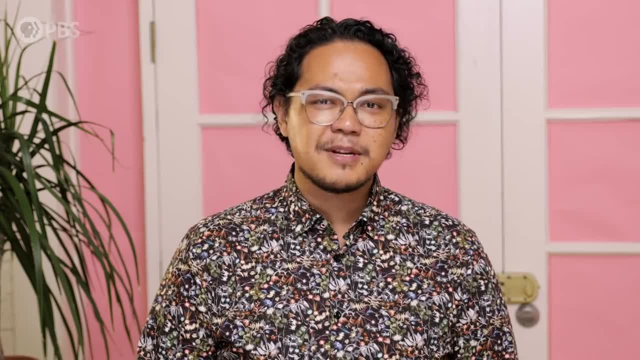 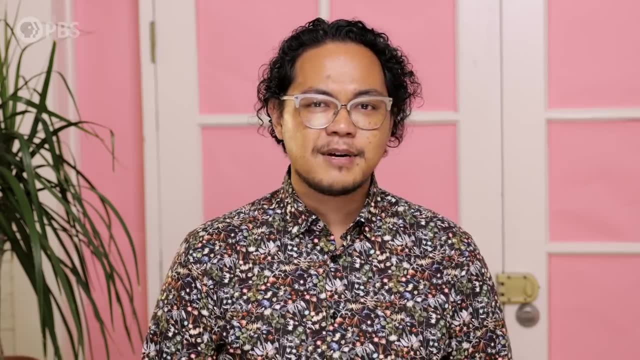 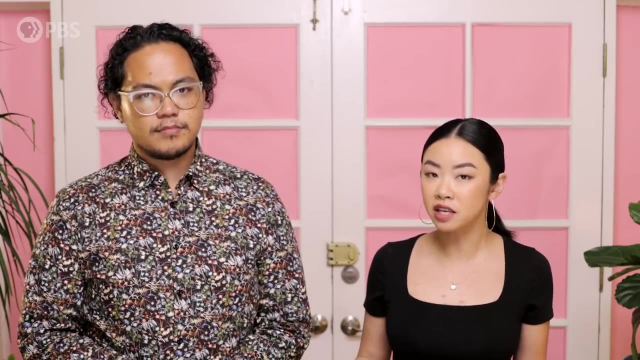 of identity and ancestry and, most importantly, to remind you that the US has a history of colonization that impacts how I talk about myself too. I can see how knowing this history of colonization makes you very weary of things like nationality or neat identity labels, And, as for months like this one. 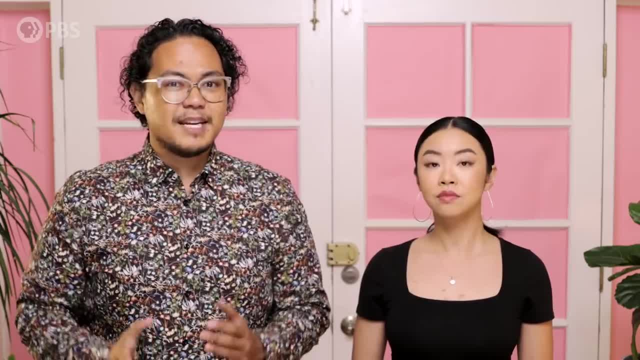 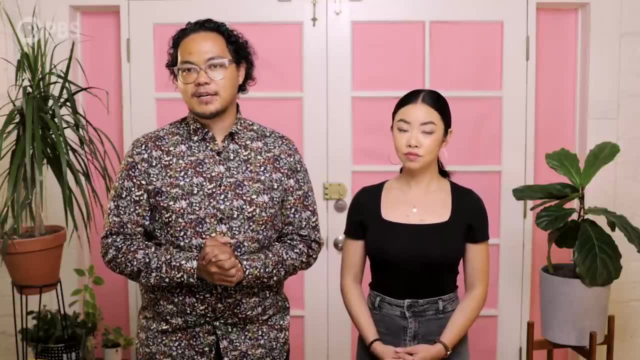 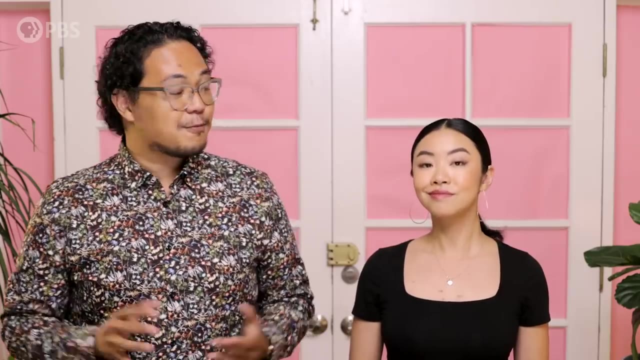 for me, these commemorations are important, but even more important is sustained curriculum. Now going back to what I mentioned earlier about ethnic studies not being taught in Canada, That's one thing that drew me to the US to become an ethnic studies professor. See, it was a pretty radical thing that. 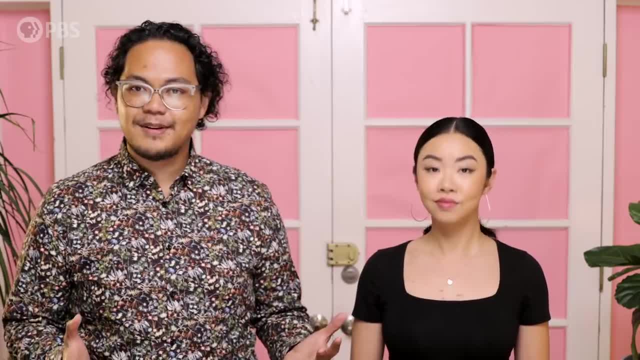 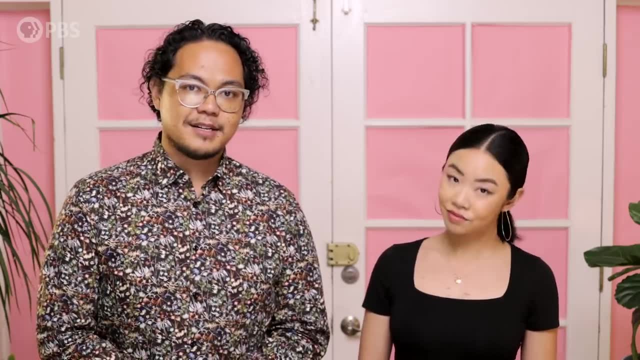 in the US, they didn't teach you about ethnic studies. This field was created out of activism, and it was radical too that Asian American identity was first and foremost created as a political identity. And well, even the name of our show, A People's History of Asian America, is. 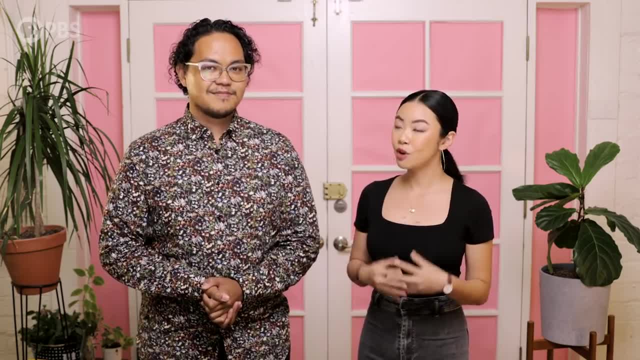 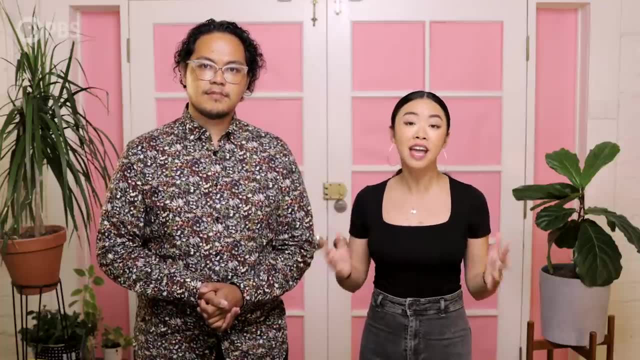 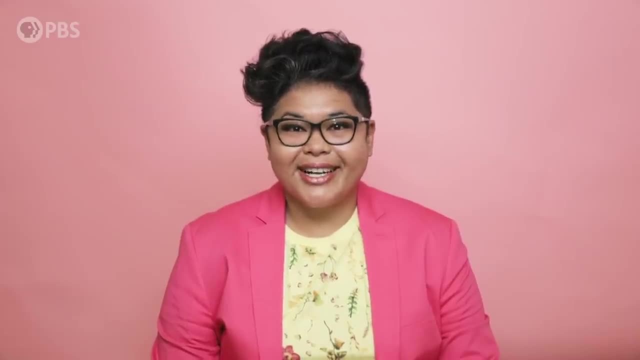 really about the political identity of this community, which is why it's so important for us to discuss the history, evolution, pros and cons of AANHPI Heritage Month. I feel like this month tokenizes my community. I've never been asked to do so. 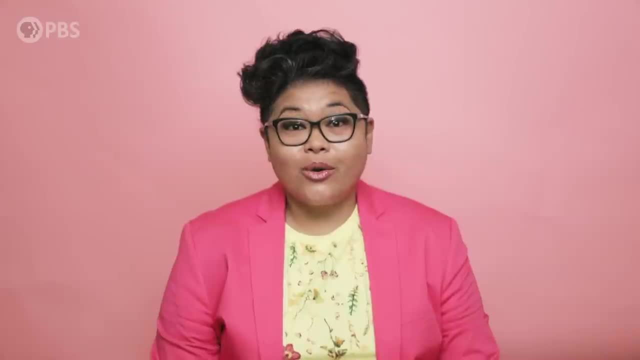 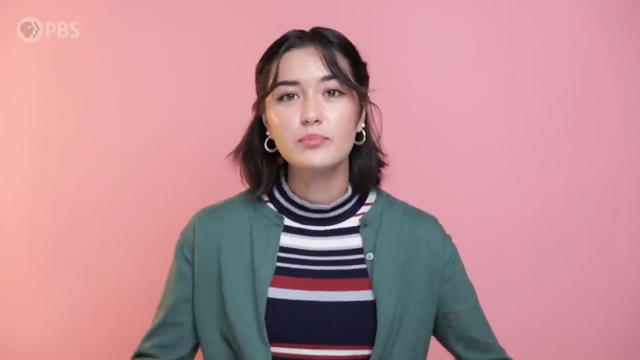 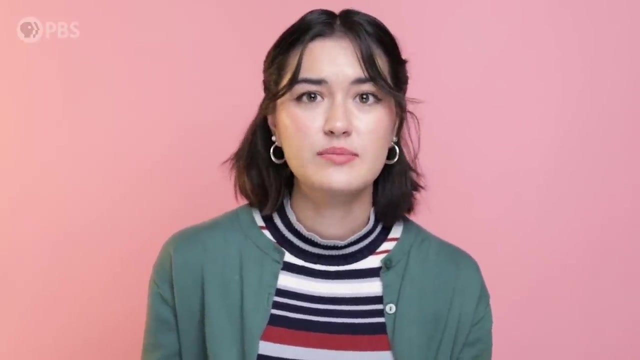 many things and I also wonder about where will we be next month. Do I feel like this month belongs to me, like and my people? No, not really. Sometimes it just feels a little shallow to me and, in addition to like Black History Month, it's like why do we need to designate a certain box of? 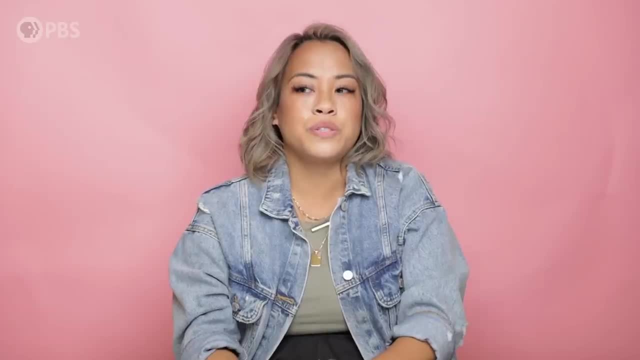 things for people of color to exist in. We don't just want a seat at the table, we want a voice at the table. We don't want to be the diversity hire. You don't want your face paraded out there as the Asian American face. You want to be the Asian American voice and you want to be 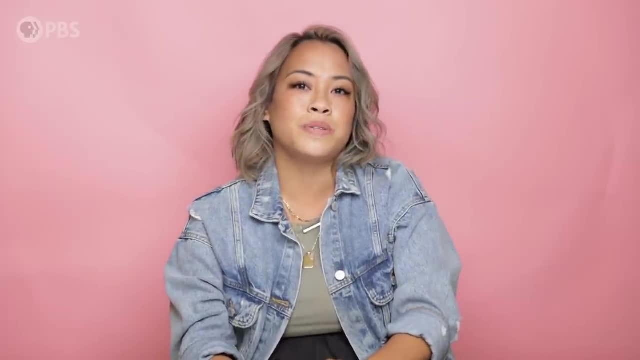 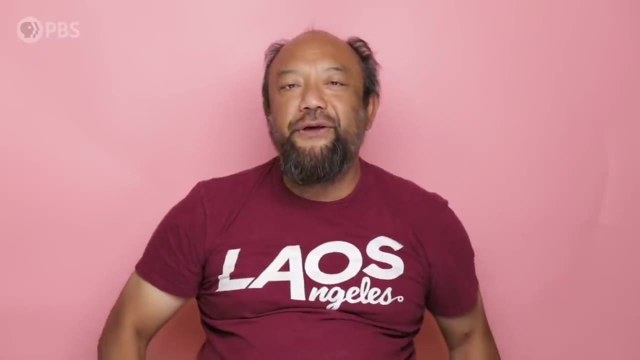 able to bring others up with you. So I think inclusion, as opposed to representation, is to say we, we are powerful, we have a voice and we want to be a part of the decision-making as well. I am very hopeful for the future of 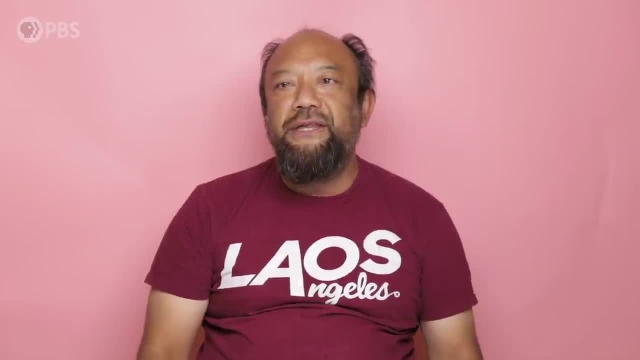 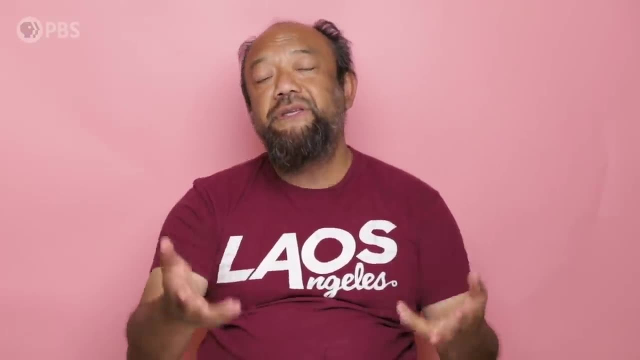 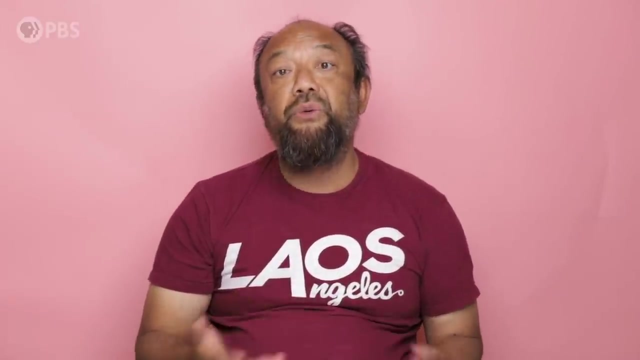 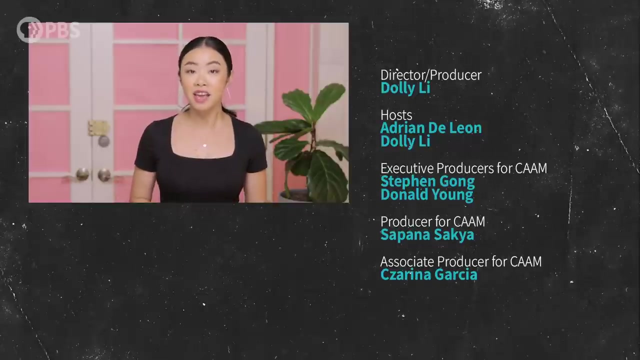 Asian America of Native Hawaiian recognition of Pacific Islander, multiple identities. When we uplift each other and support each other and connect with each other and cross-culturally do that, I feel we rise together. So what do you guys think about using AAPI, APIDA, APA, AANHPI or Asian? 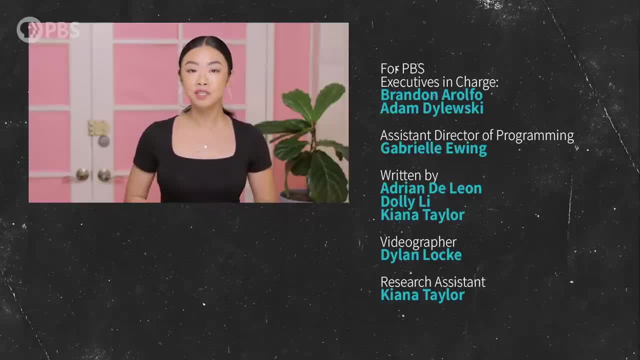 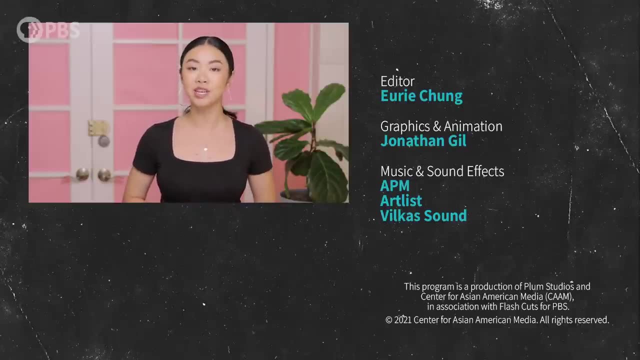 American. Which terms have you heard and which one feels most inclusive to you? Tell us in the comments below and make sure you tune in next week for another episode of People's History of Asian America. This episode was made possible by the Corporation for Public Broadcasting. Thank you.